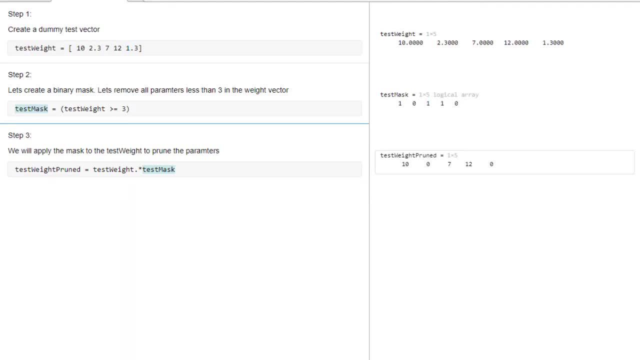 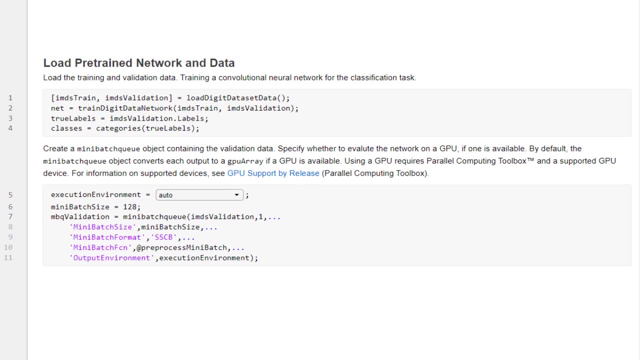 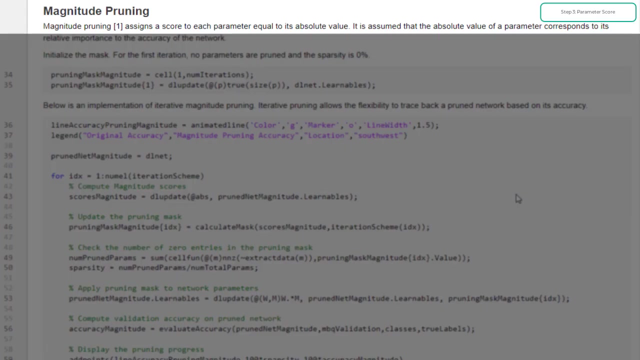 Beware: this technique creates sparse matrices and will not provide any size or computational gain. Here we load the training and validation data and train a recombination neural net to classify handwritten digits as the network subject to pruning. For pruning we need to assign a score to each parameter. 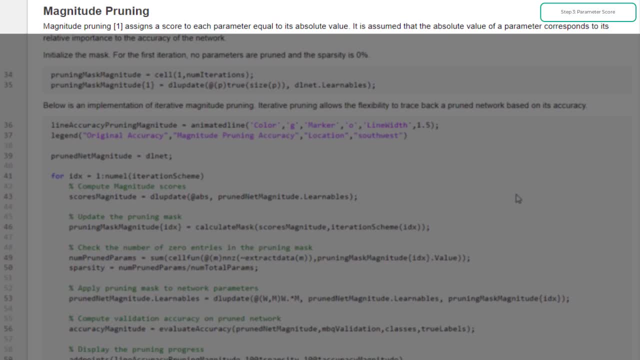 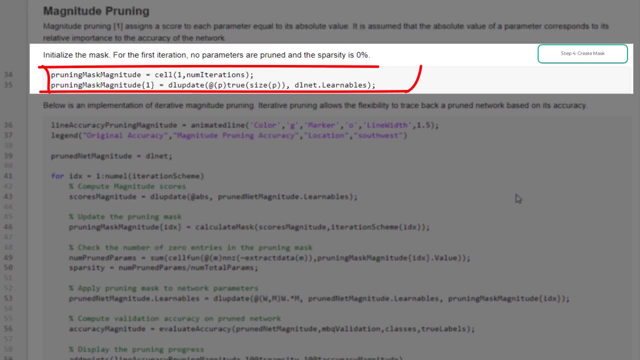 which decides its importance. For magnitude pruning, the absolute value of the parameter is considered the score. The next step: we create a network mask for each iteration. This helps us trace back the best solution. The first step in the loop: we create the magnitude score. 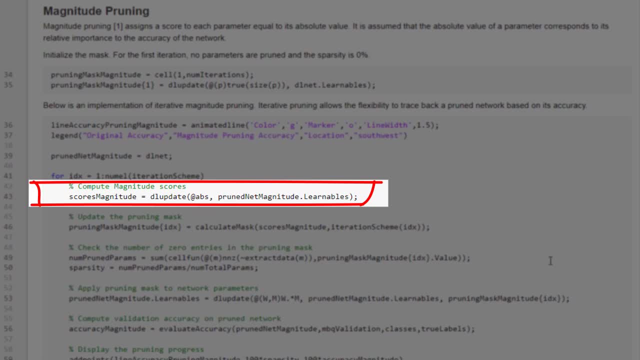 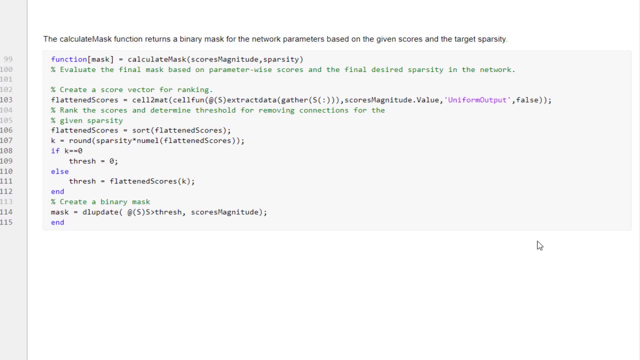 Then this score is used to create the iteration mask. For the iteration mask the score is packed into one vector to calculate the minimum threshold score value for the given iteration sparsity. The mask is then created to prune all parameters with scores below the specific threshold. 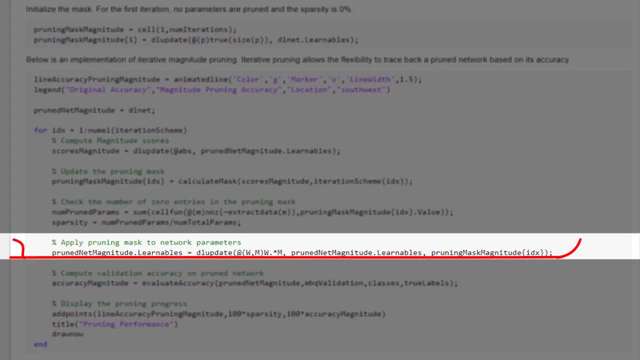 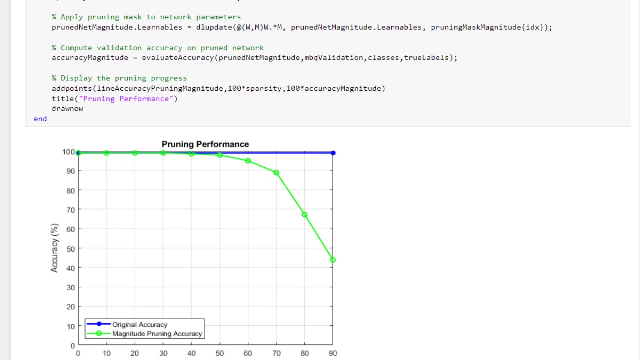 Once we evaluate the iteration mask, DL update is used to update the network learnables. The pruned network is used to calculate the iteration accuracy. Now these accuracy metrics are compiled to have a plot between the sparsity versus the network accuracy, which can help us trace back the best solution. 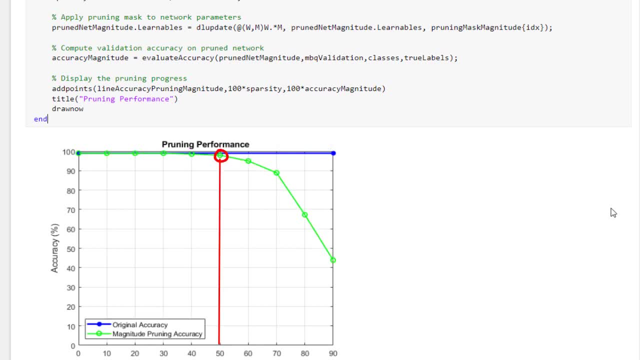 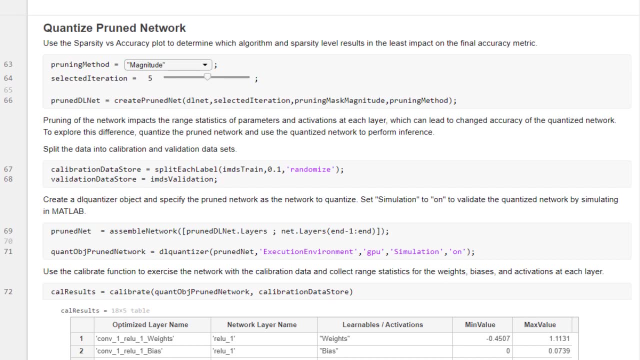 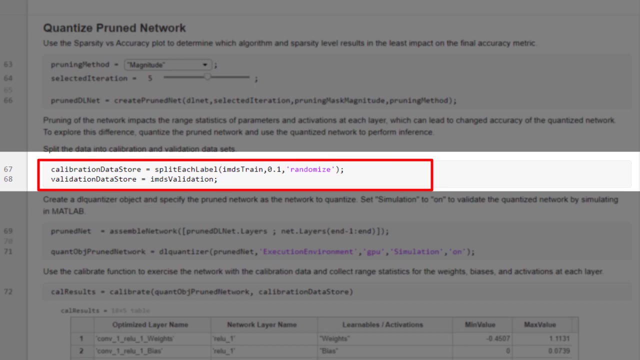 which in our case is, we can prune up to 50% of parameters for 1% accuracy loss Once we have the pruned network. now we will quantize the pruned network using the model quantization library. First we need to create a calibration and validation data store. 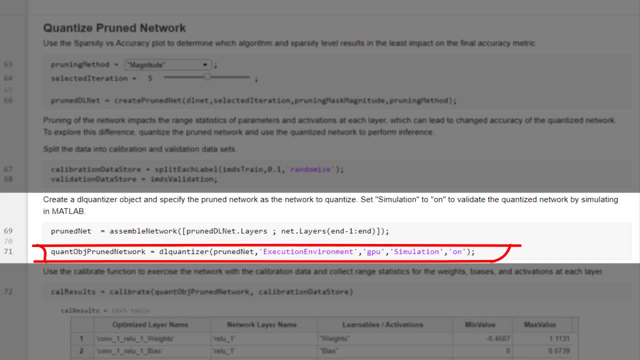 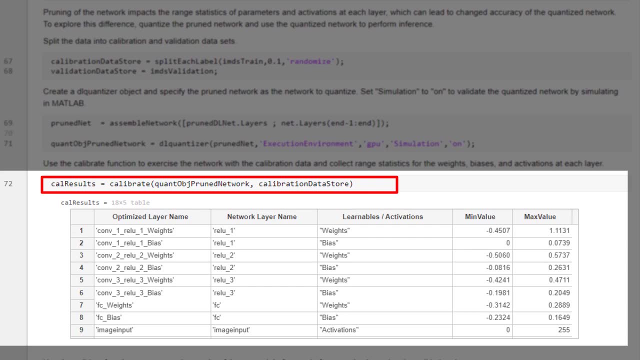 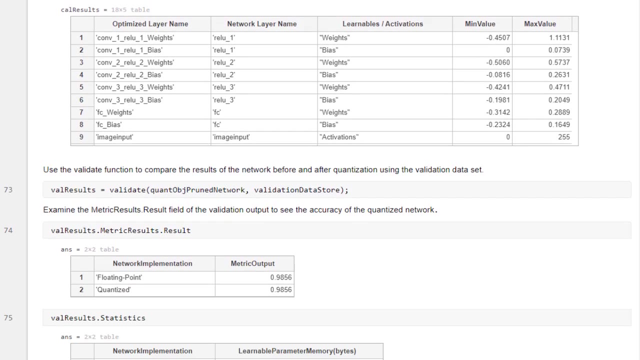 We then create a DL quantizer object for the pruned network. Next, we calibrate the quantizer object to collect the range statistics for the weights and activations. Once the calibration is done, we can validate the quantizing behavior using the validate step. 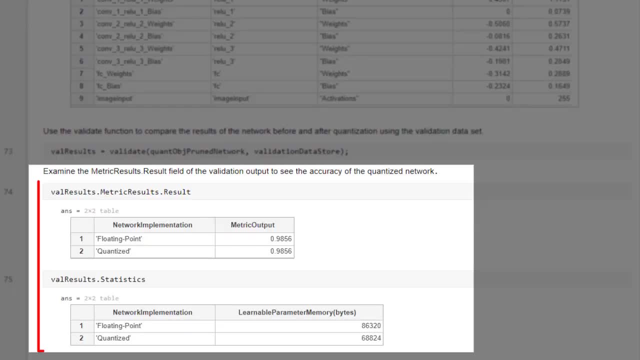 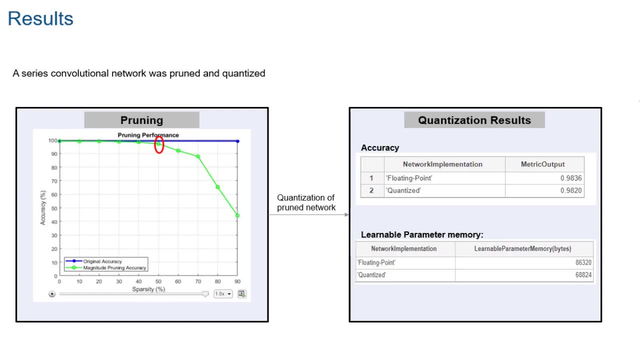 to get the accuracy and the learnable parameter memory for the floating point and quantized network. Pruning and quantization was applied to a network trained to classify handwritten digits. We could achieve up to 50% pruning with less than 1% accuracy loss. 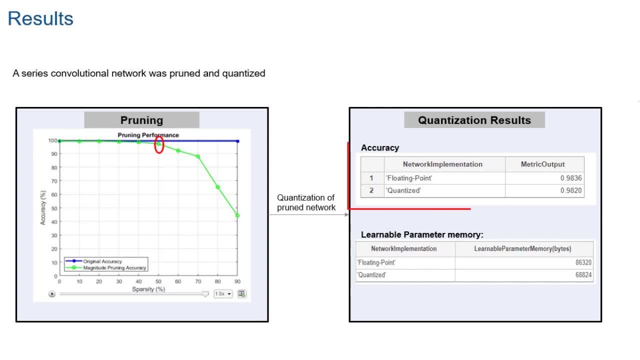 and the quantized network had little to no accuracy loss compared to floating point network.